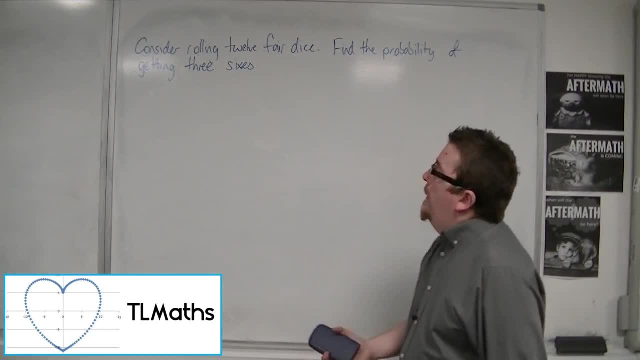 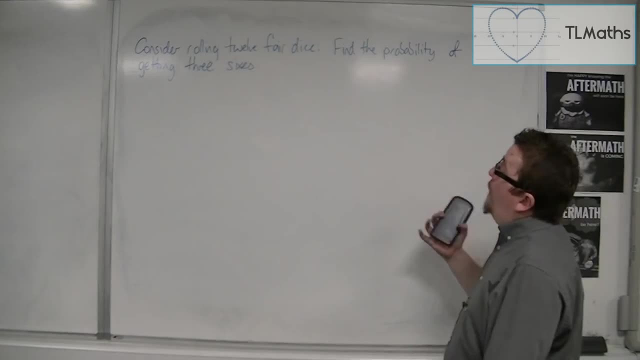 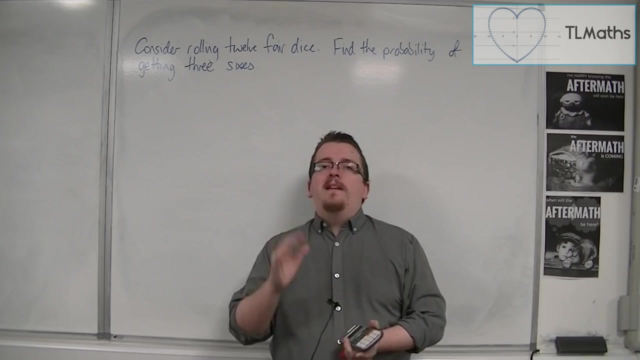 So, carrying on from the previous video, let's make it a little bit more tricky. Consider rolling 12 fair dice. Find the probability of getting three sixes. Now, if we relate it back to the previous problem, this would be like drawing out a probability tree with 12 branches, 12 stages. 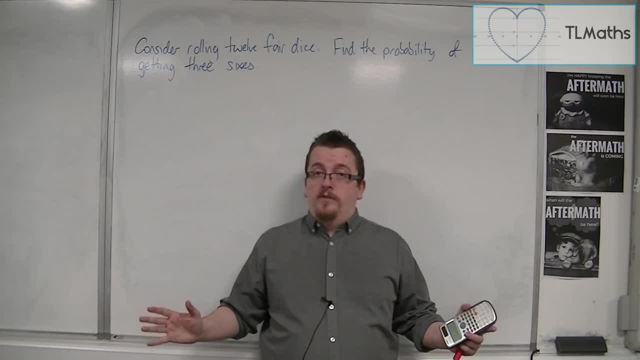 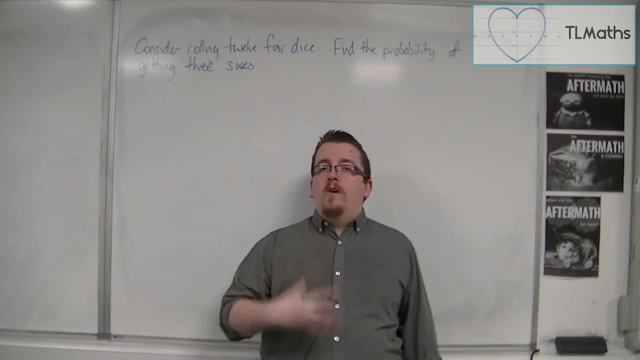 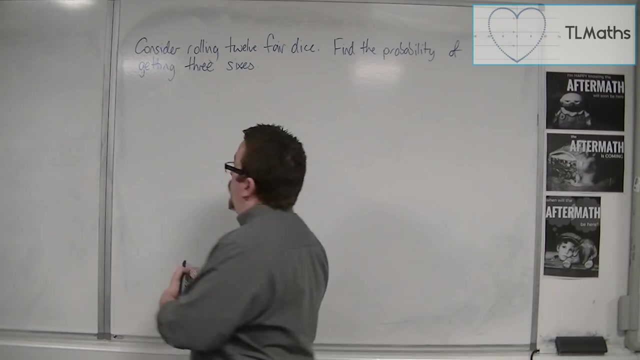 Now that is going to fill the board okay and would be very complicated to work with, But the pattern that we were writing down from last time will enable us to find this probability. So we want the probability of getting three sixes. 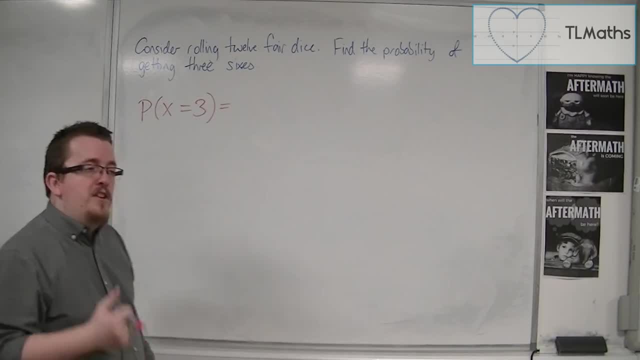 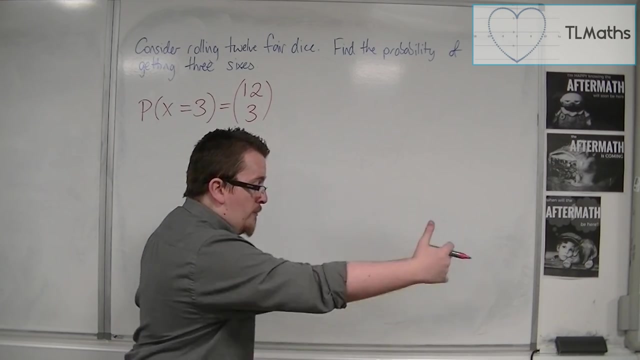 So we first of all want the number of ways of So choosing three sixes out of the 12.. So 12 NCR 3.. So this is actually finding going down to the 12th row of Pascal's triangle and then going in 1,, 2,, 3.. 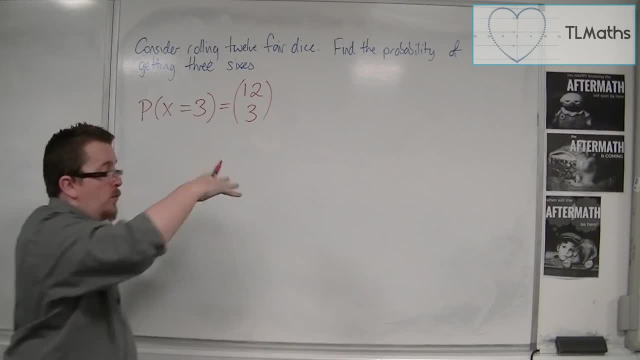 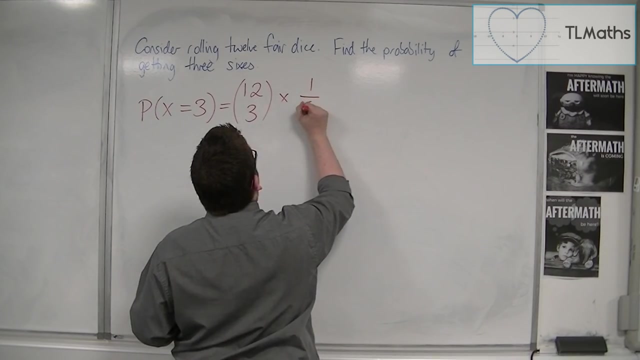 And that would give. this is giving me the number in Pascal's triangle all the way at the bottom there. okay, Now I I want a 6 to appear three times. So the probability of a 6 appearing is 1- 6th and I want that appearing three times. 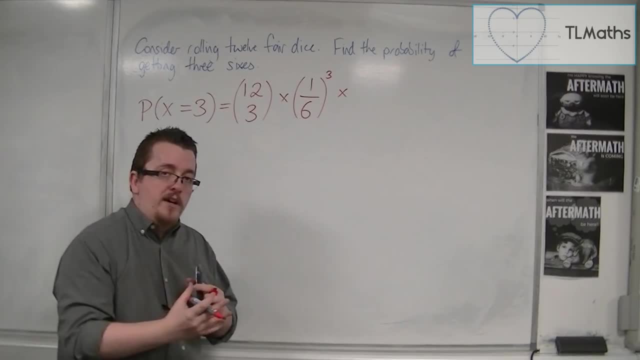 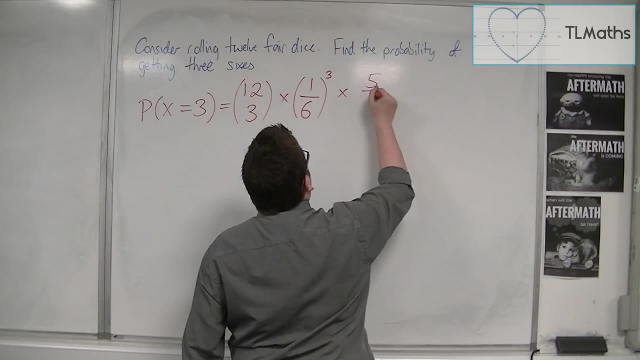 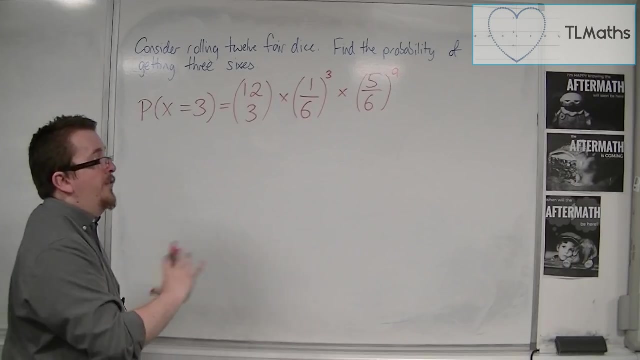 And subsequently, because the 6 is appearing three times, not a 6, is appearing nine times. So 5, 6th is getting multiplied nine times. okay, So 5, 6th Times, 5, 6th times, 5, 6th times, 5, 6th. 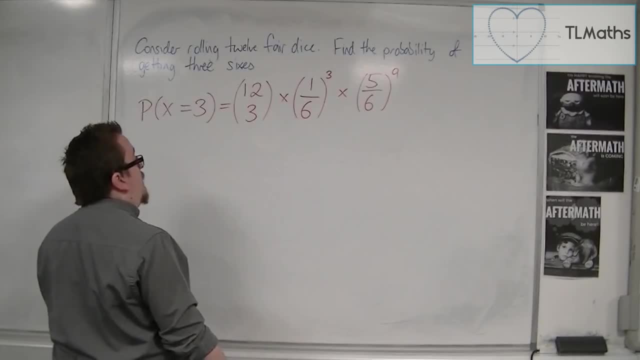 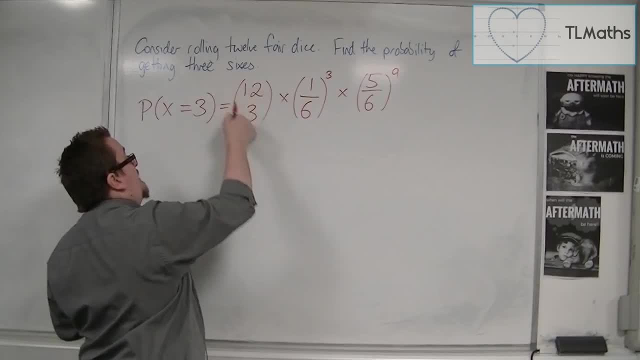 And that's just one branch And this is how many branches I would need to add together. So 12, choose 3.. So 12 NCR 3 is 220. So there'd be 220. So there'd be 220 branches effectively that I would need to add together. 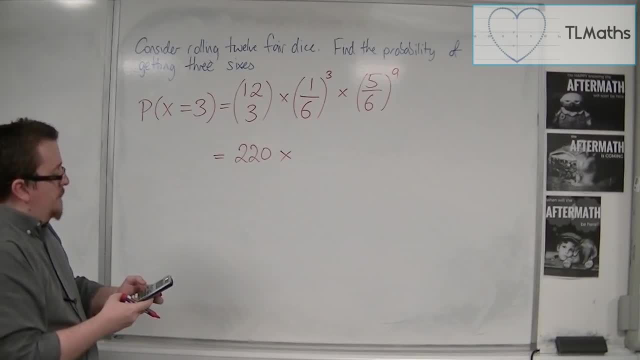 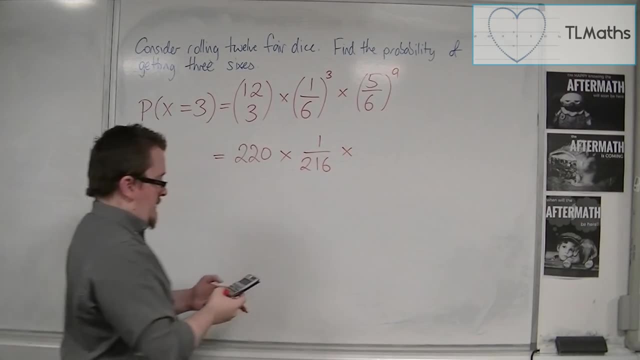 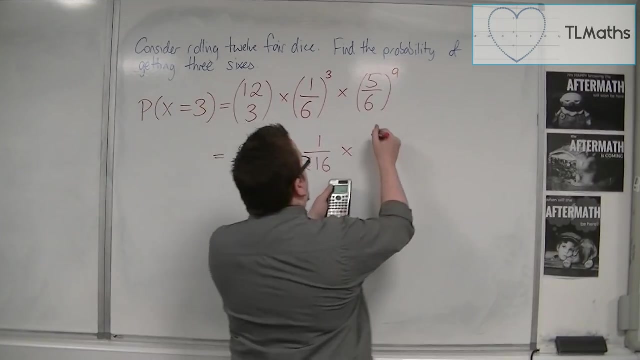 Times by 1 over 6 to the power of 3,, which is 1 over 216.. Now I don't think my calculator's going to give me this as a nice number, which it's not. So 5 to the power of 9 is 1, 9, 5, 3, 1, 2, 5.. 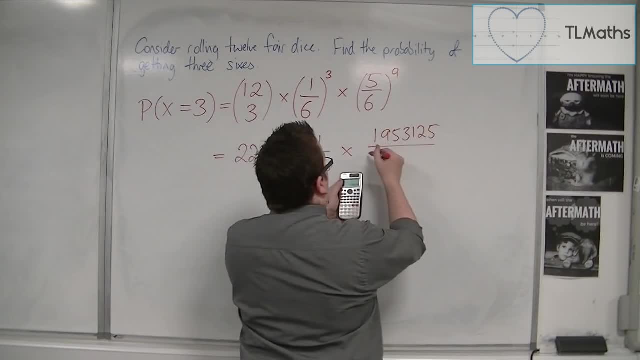 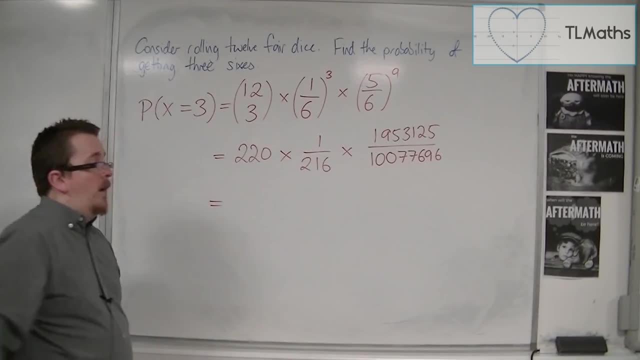 And 6.. 6 to the power of 9 is 1, 0, 0, 7, 7, 6, 9, 6.. Okay, Now, I personally would put this all into the calculator in one go from this line, okay. 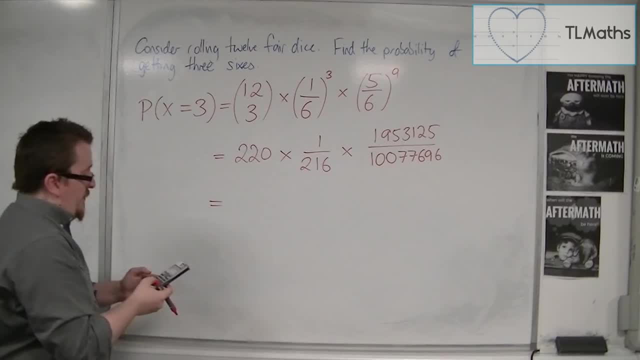 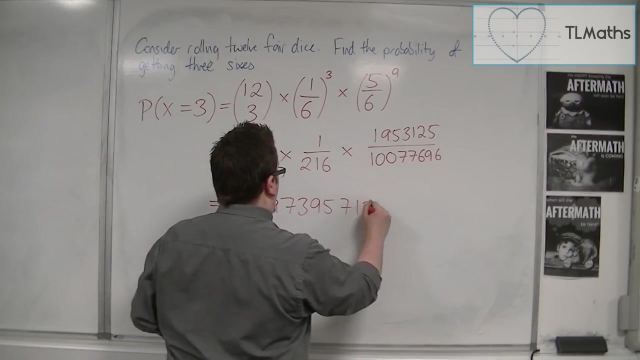 But I wanted to show you the separate pieces here. So we have 12 NCR 3 times by 1 over 6, cubed, And then times that by 5 over 6.. So 1 over 6 to the power of 9, which is actually 0 point 1. 9, 7, 3, 9, 5, 7, 1, 2, 4.. 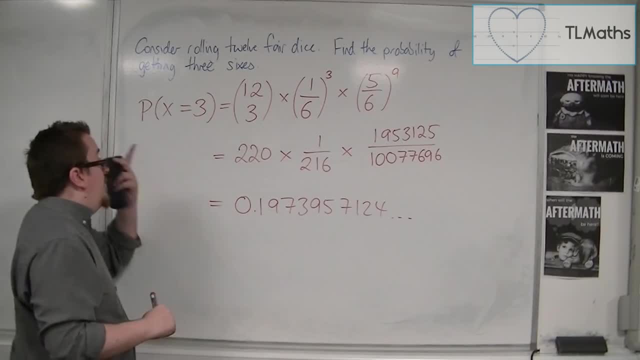 Now does this as a probability make sense? Now, if you think about it, if you're rolling 12 fair dice, then you would probably expect a 6 to appear twice, So 1 sixth of the times. So 12 times 1 sixth is 2.. 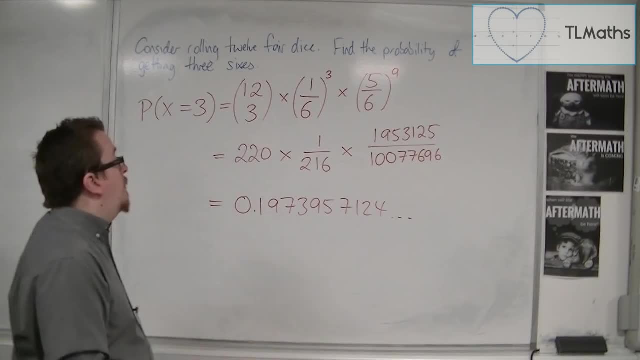 So you'd expect it to appear twice. So the probability of getting 3- 6s, that seems fairly reasonable. Okay, You wouldn't be surprised, in other words, if 3 6s appeared or 1 sixth. 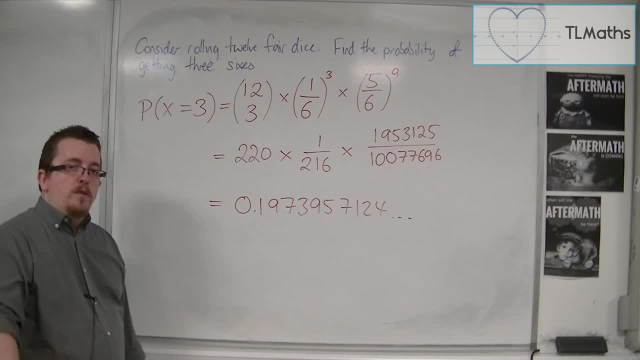 But if 12- 6s appeared, you would be quite surprised. Okay, So that doesn't seem fair Far off what you would expect in this case. Thank you,